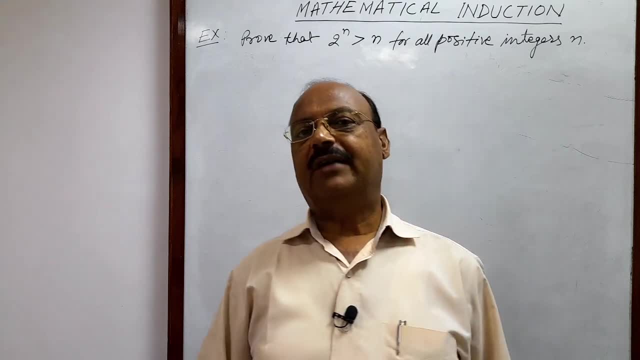 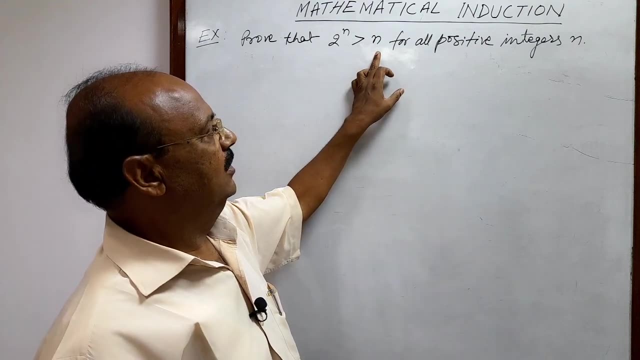 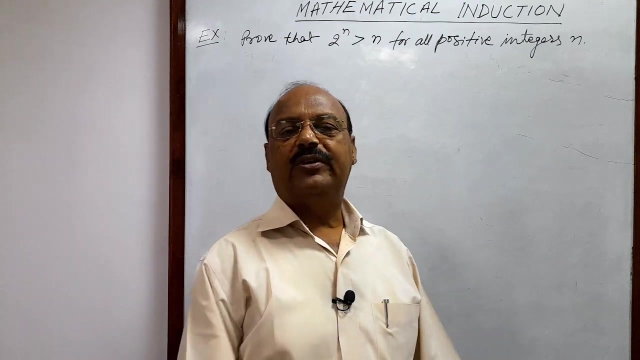 Welcome students. Let us see a very interesting and important question from the chapter Mathematical Induction Here. question is: prove that 2 to the power n is greater than n for all positive integers n. So we have discussed so many questions from the same topic and you know. 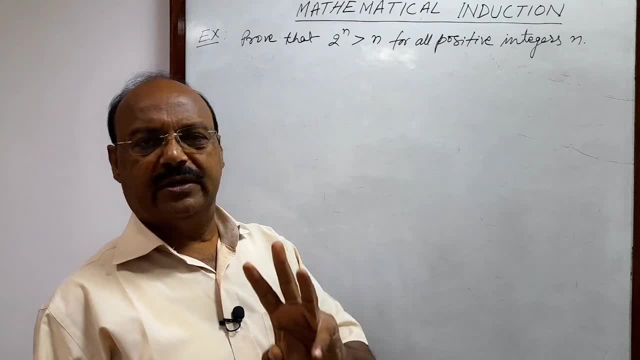 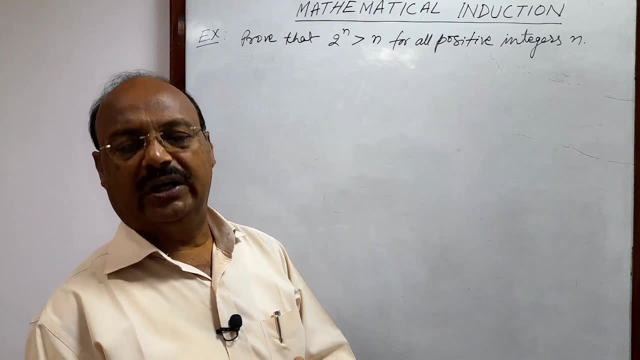 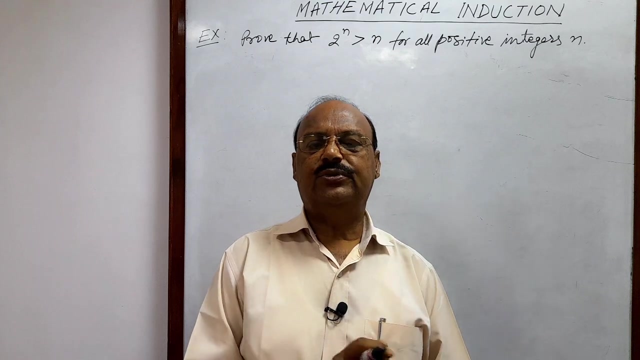 that we can solve it very easily using three steps only. In first step, we have to show that this statement is true, for n is equal to 1, first step. Second step: we assume that this statement is true, for n is equal to r. I mean p r is true. And third and final step. 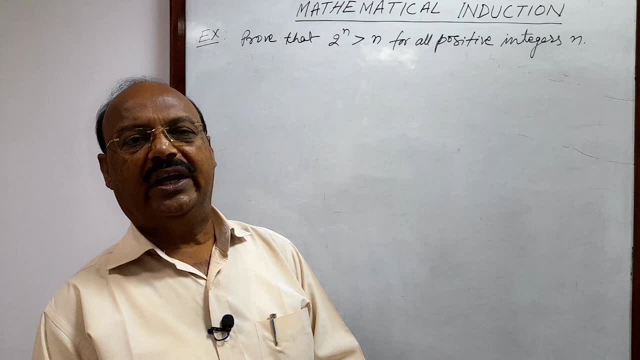 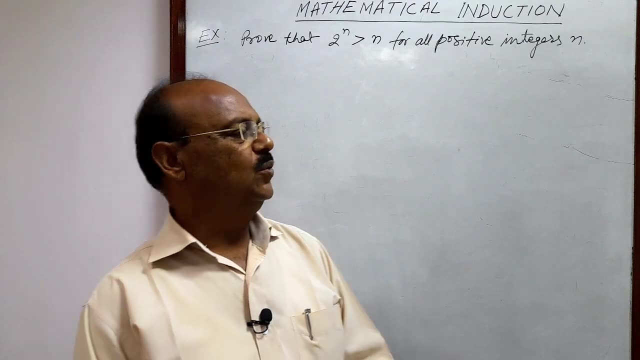 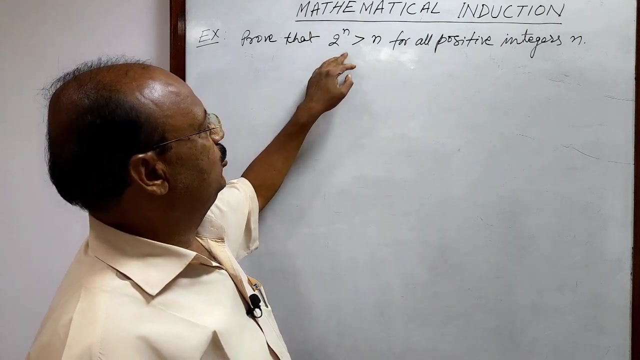 we show that this statement is true, for n is equal to r plus 1, means p r plus 1 is true. So by that we can conclude that the given statement is true, for n is equal to 1.. So this is the mathematical statement for all n. Here mathematical statement is 2. 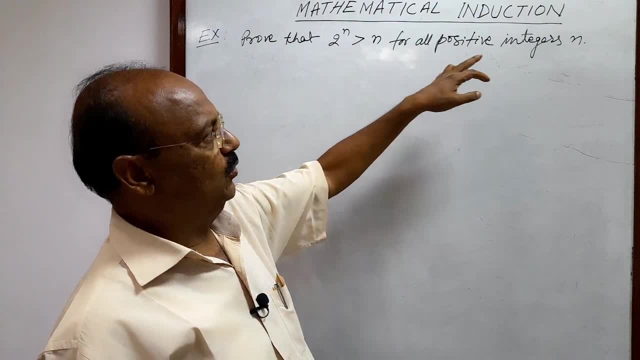 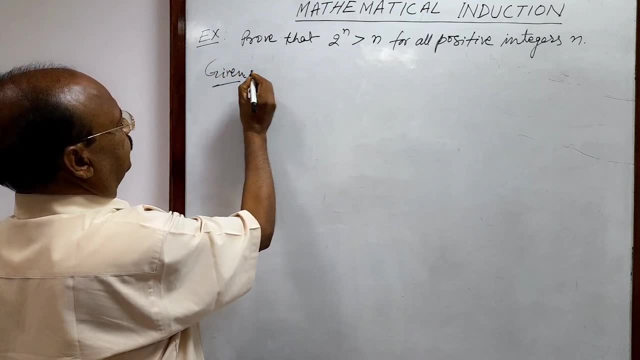 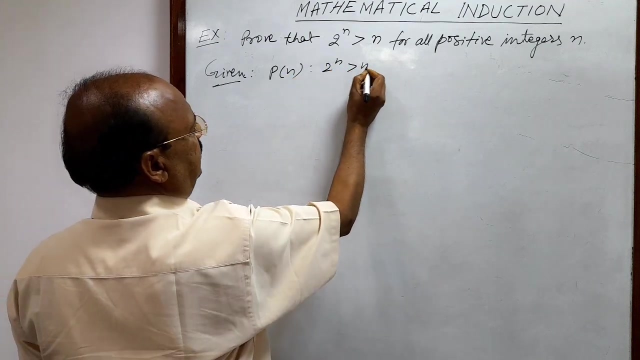 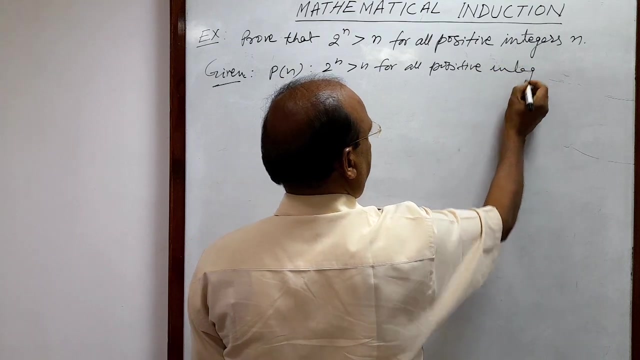 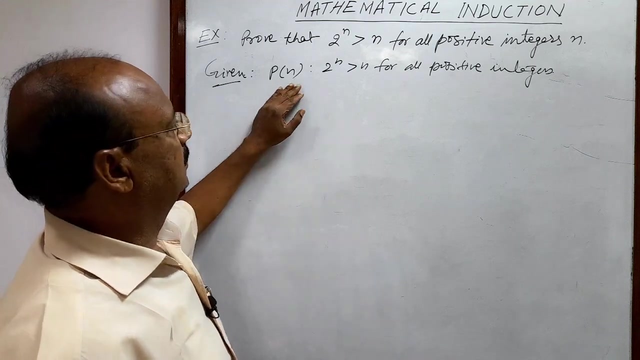 to the power n greater than n for all positive integers, and mathematical statement is denoted by the notation p n. So here p n is 2 to the power n is greater than n for all positive integers. okay, so first step, we have to show that p1 is true. let us write it: relation. 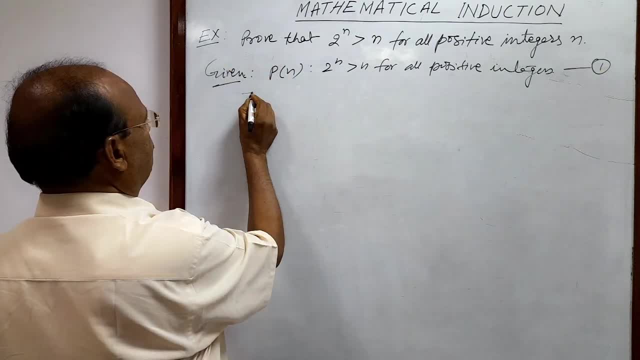 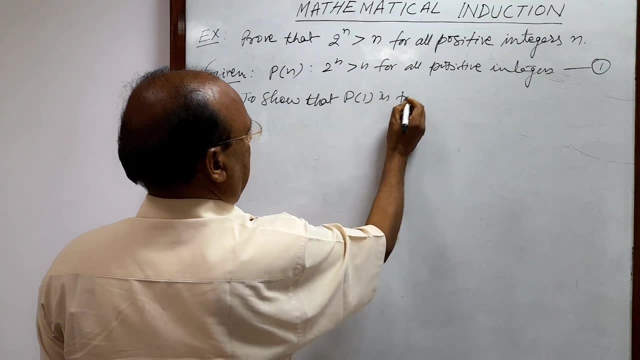 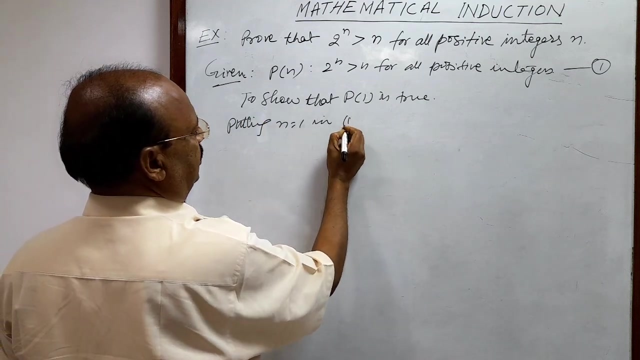 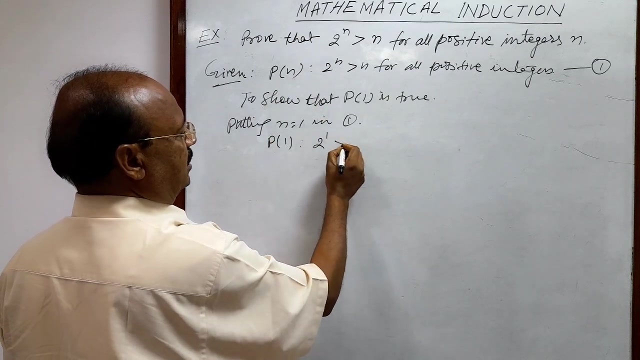 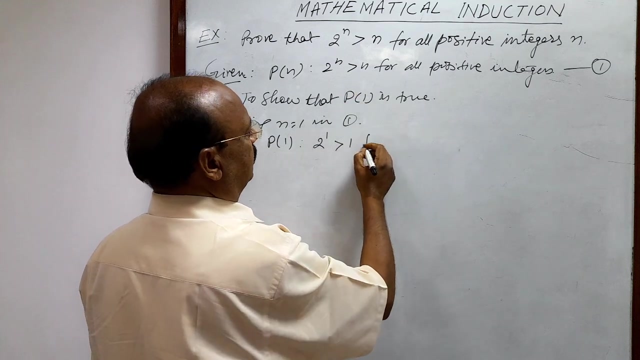 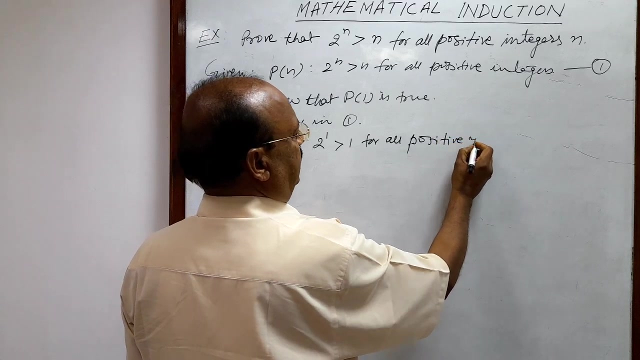 number one. so here we have to show that, to show that p1 is true. so putting n is equal to one in relation number one. okay, so here p1 will be two to the power, one is greater than one, which is true. so this is true, it must be true for all positive, all positive integers. 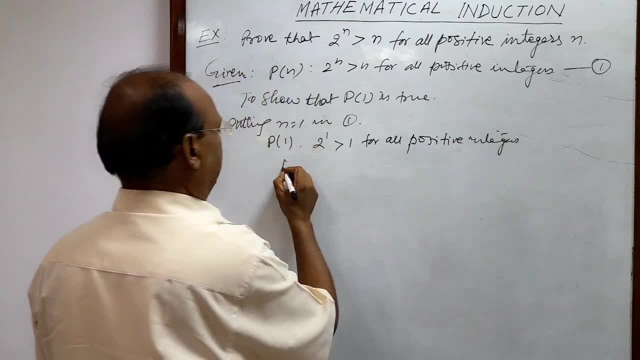 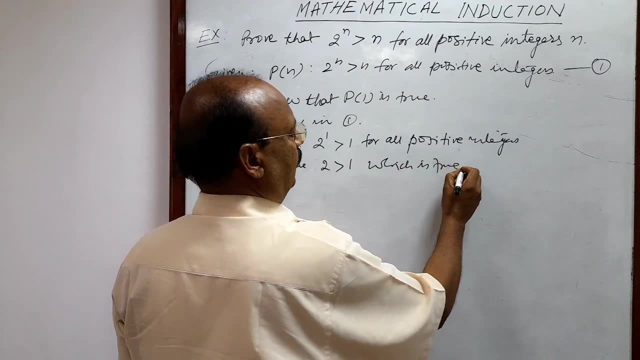 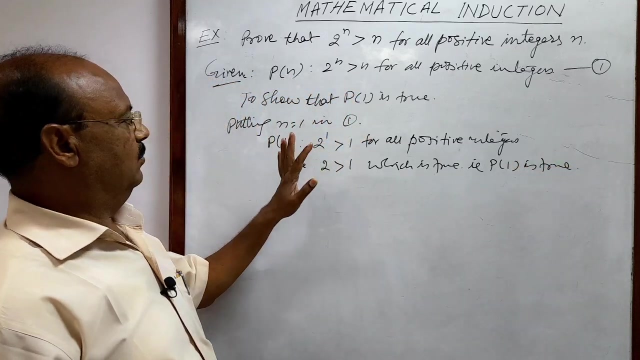 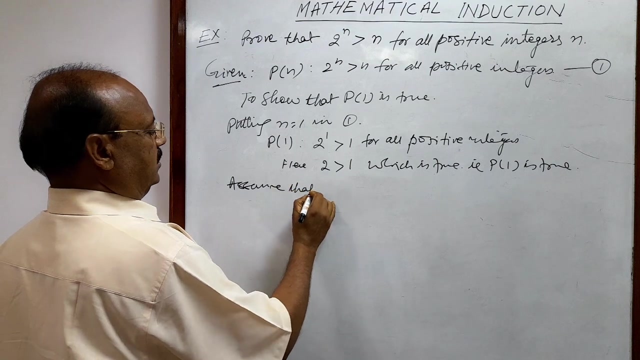 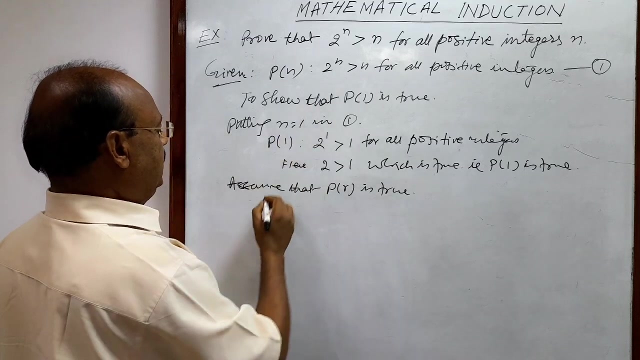 so here we find that two is greater than one, which is true. that is, p1 is true. okay, so our first step is complete. now second step: we assume, we assume that PR is true. okay, so PR means putting n is equal to R. okay, so PR means putting n is equal to R. 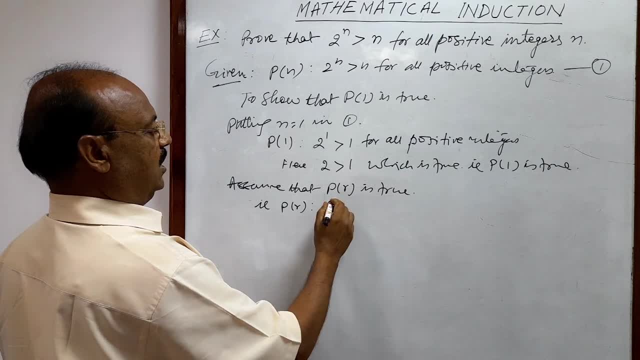 okay, so PR means putting n is equal to R. so that is two to the power. sorry put. so that is two to the power. sorry put. so that is two to the power, sorry put here. R 2 to the power R is greater than here. R 2 to the power R is greater than. 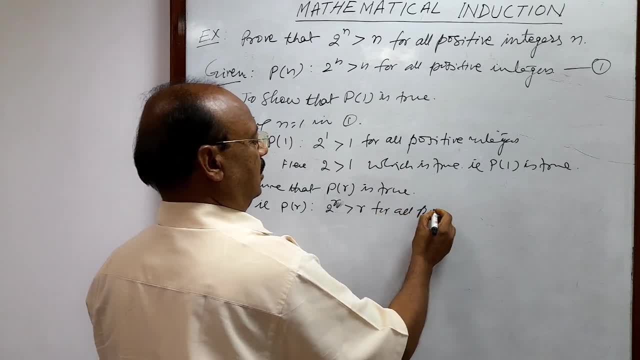 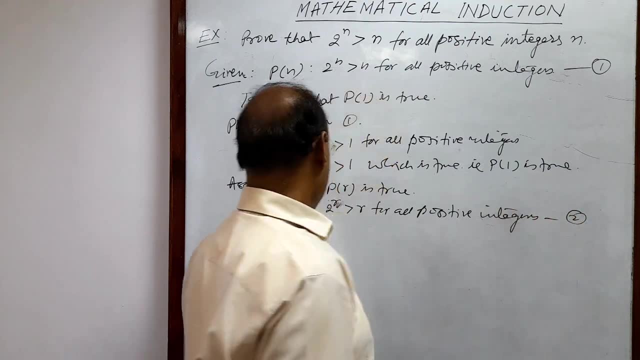 here R 2 to the power R is greater than R for all positive integers. suppose this R for all positive integers. suppose this R for all positive integers. suppose this is relation number two. so we are is relation number two. so we are is relation number two. so we are assuming that this relation is true PR. 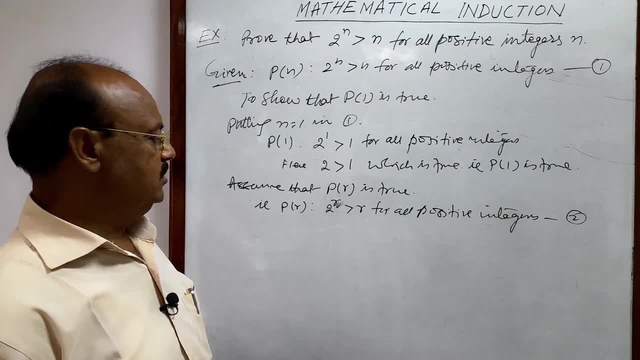 assuming that this relation is true, PR, assuming that this relation is true, PR is true. and third and final stage, last is true. and third and final stage, last is true. and third and final stage, last stage. we have to show that PR plus one stage. we have to show that PR plus one. 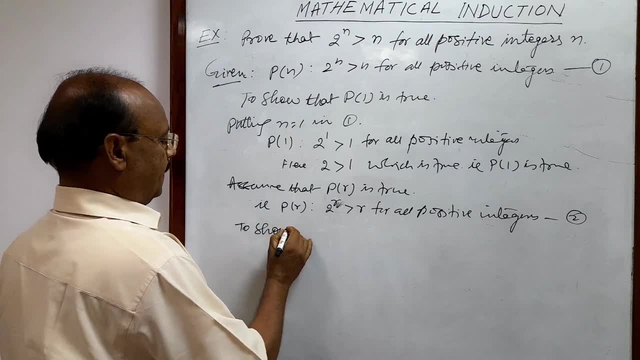 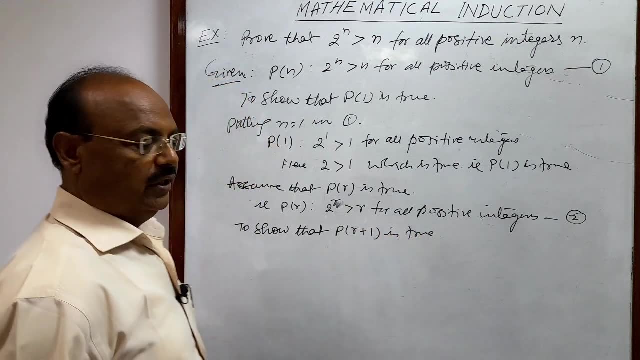 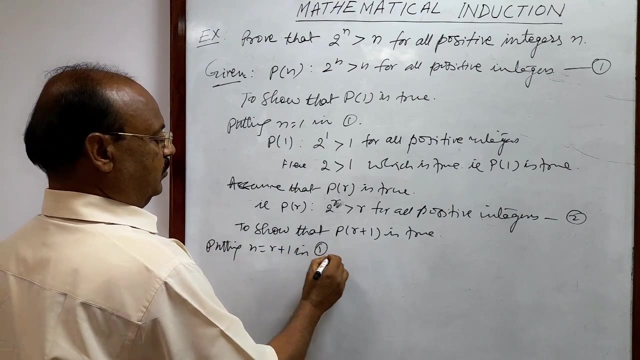 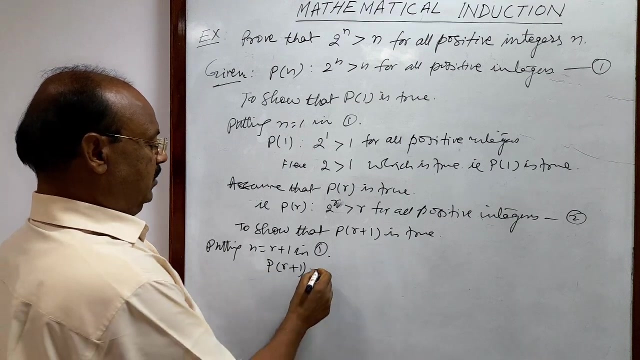 stage. we have to show that PR plus one is true. now we have to show that. we have to show that p r plus 1 is true. ok, so putting n is equal to r plus 1. in relation number 1, we will get p r plus 1. this statement: p r plus 1 will be 2 to the. 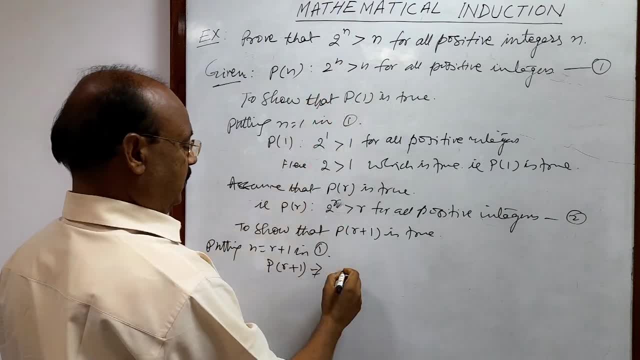 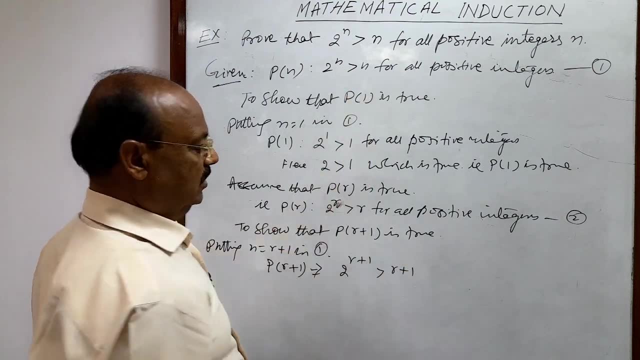 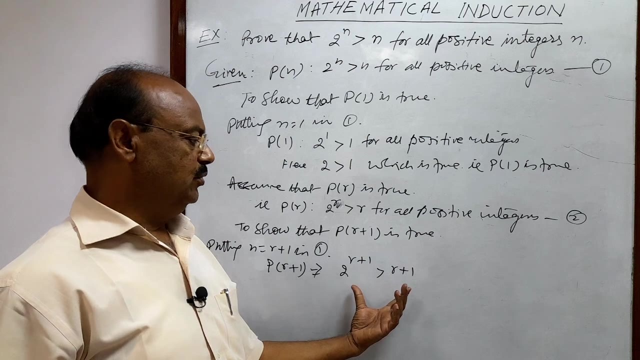 power n. so n place of n, we have to write r plus 1, 2 to the power, r plus 1 is greater than n. place of n, you have to write r plus 1. so we have to establish, we have to show that this relation is true for all integers, all positive integers n ok. so we have to prove. 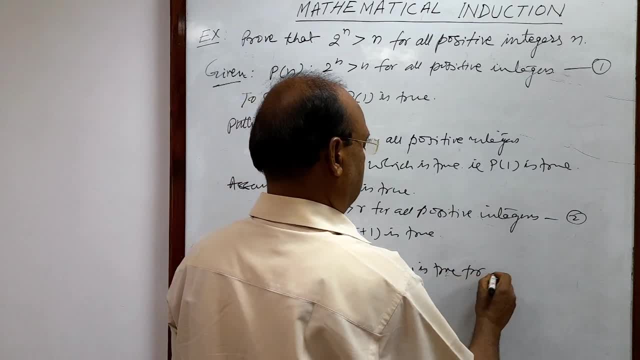 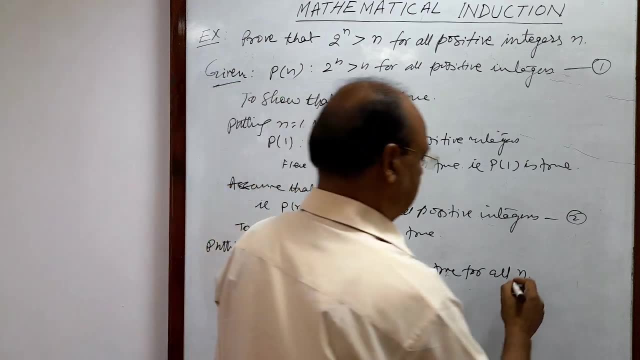 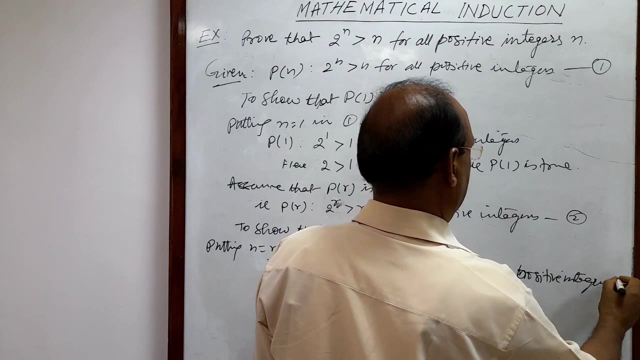 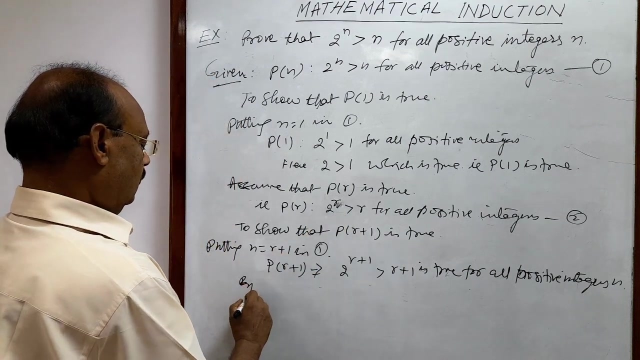 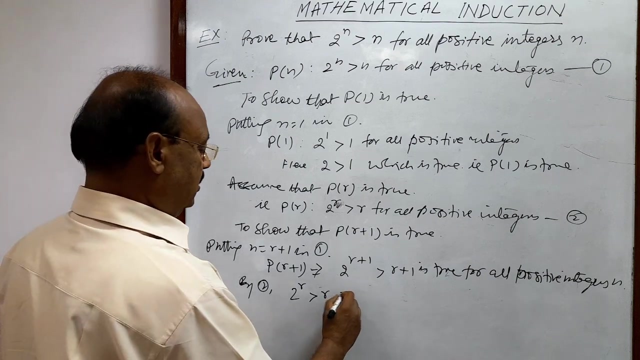 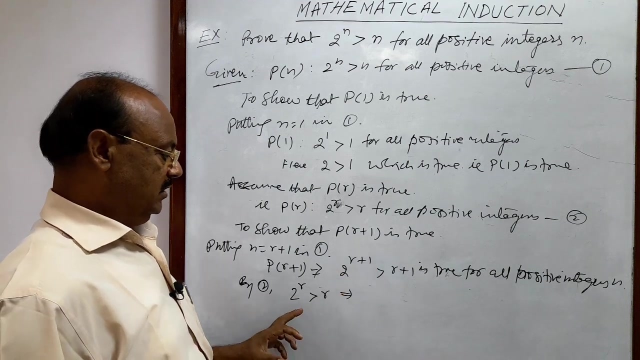 that this is true for the all positive integers n or write the completely all positive integers n. So by relation number 2 we have 2 to the power. r is greater than r Here, multiplying both sides by 2, since we have to bring here 2 to the power r plus 1.. 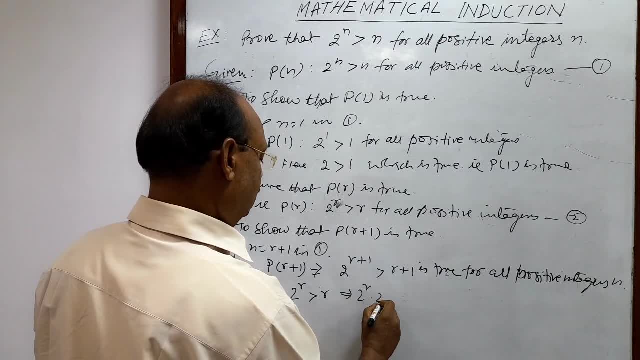 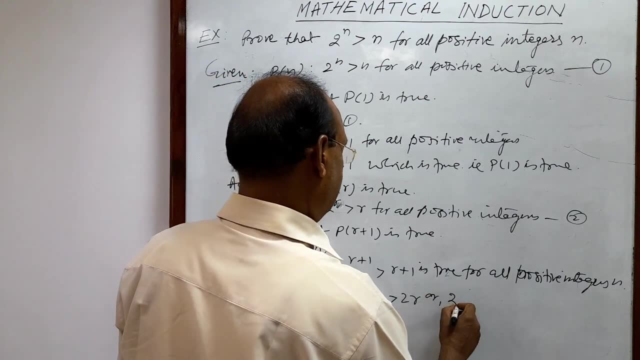 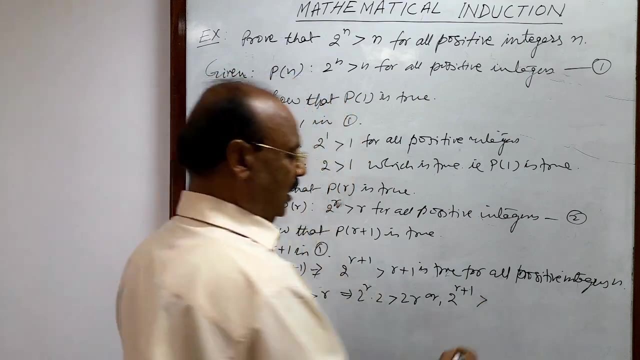 So, multiplying by 2, we will get 2 to the power r into 2.. This is greater than 2r. or we can write 2 to the power r plus 1.. This is greater than 2r, means r plus r. 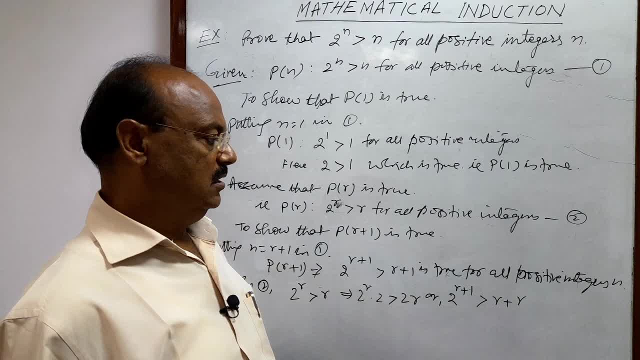 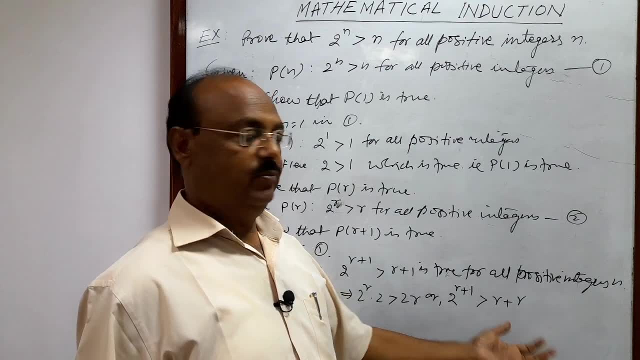 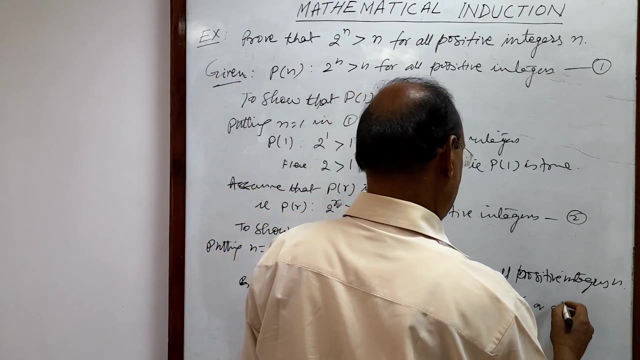 2r is r plus 2.. Or what is r here? r is also a positive integer, isn't it? In place of n we are using r, So r is also positive integer. or we can write here: 2 to the power, r plus 1.. 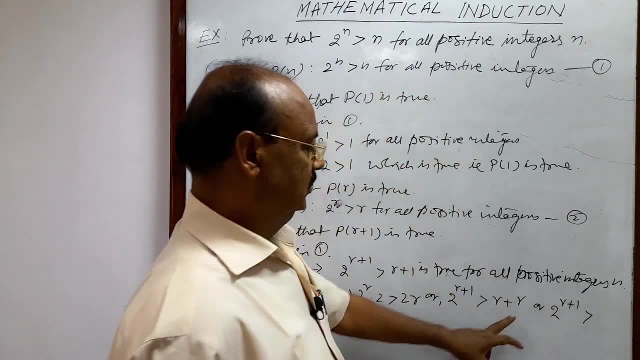 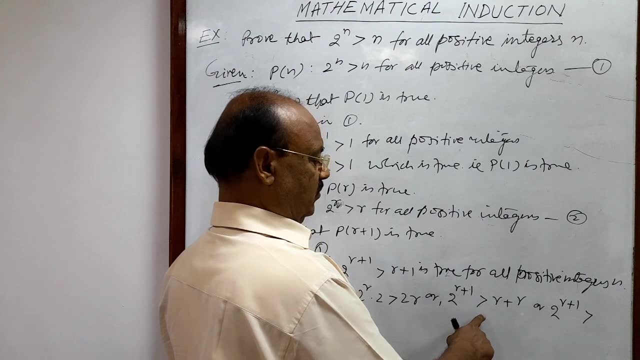 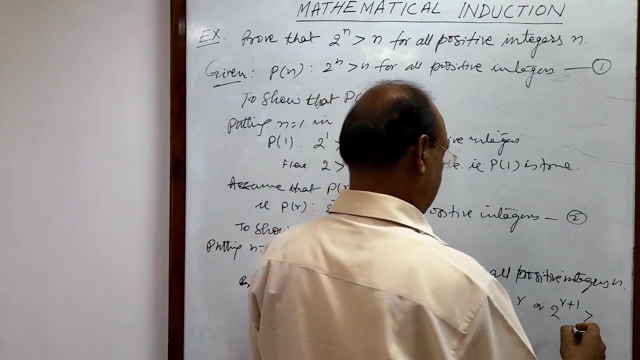 This is greater than if you put r is equal to 1. that is the first positive integer. So definitely, if 2 to the power r plus 1 is greater than r plus r, we are replacing one r by 1.. So 2 to the power r plus 1 is greater than r plus 1.. 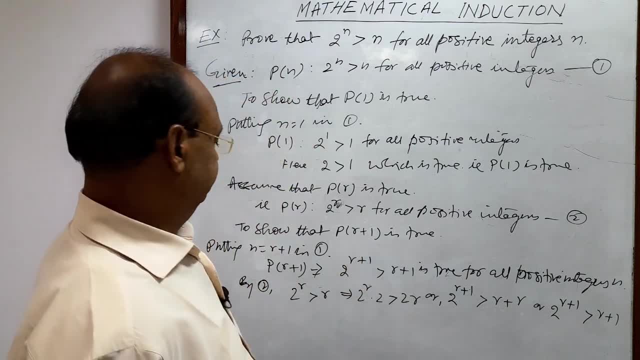 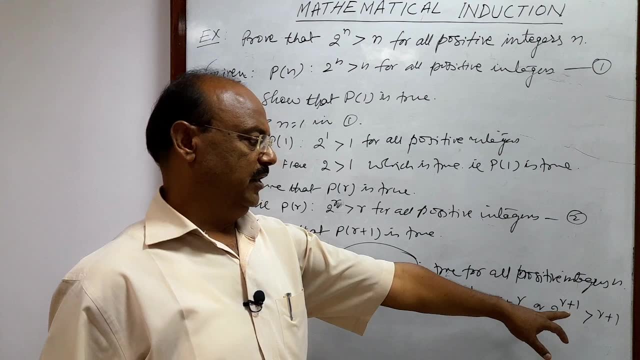 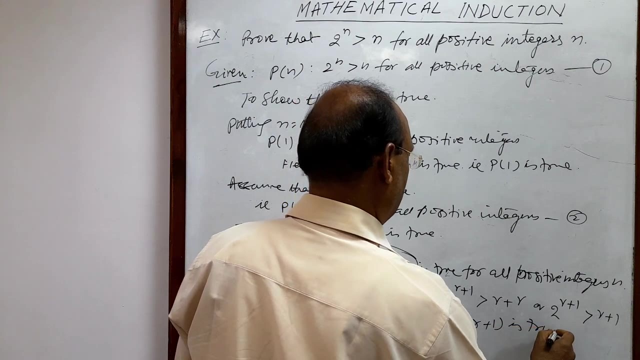 So we are getting this result here, We are getting this result, We are establishing this result, proving this result here So we can write: that is p r plus 1 is true. So this is the only three step in this problem. First step: we have to show. 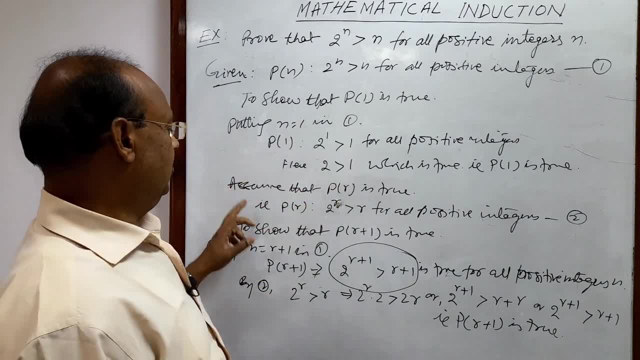 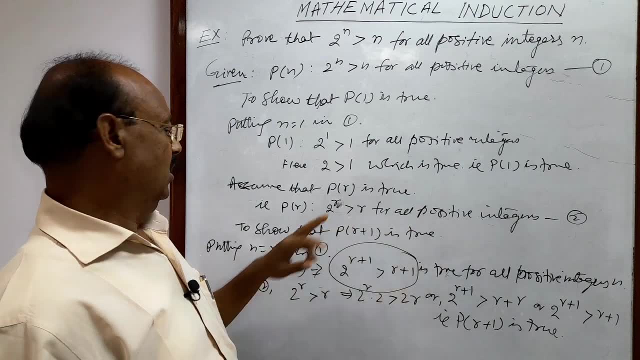 That p 1 is true, which we have done here. Second step: we assume that p? r is true, This much, This one for all positive integer is true. And third and final step, we have to show that p? r plus 1 is true.